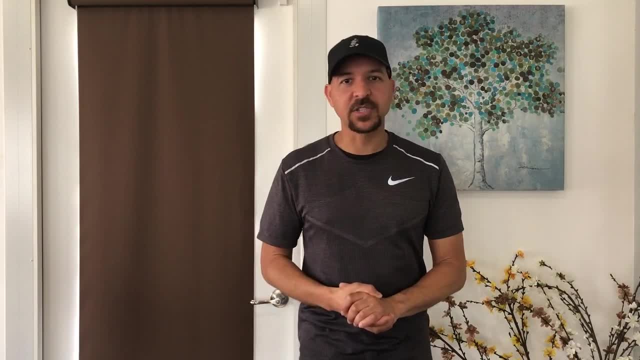 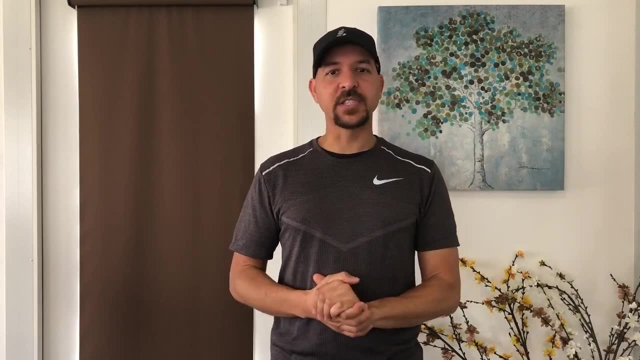 version. It's only going to take a few minutes for each example. It's going to be a quick video today. First of all, I hope everybody's staying safe and healthy and happy out there. We're going to get through this together, guys. Let's just have a little fun reading some music together. Here we go. 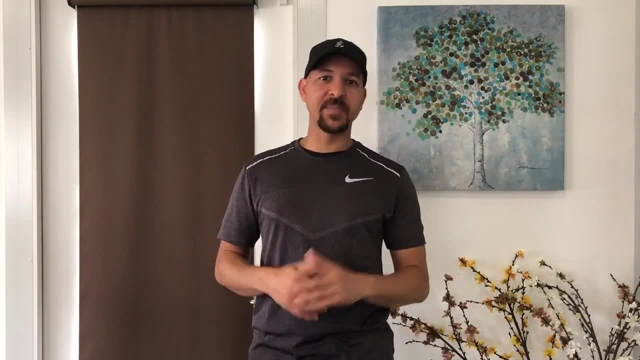 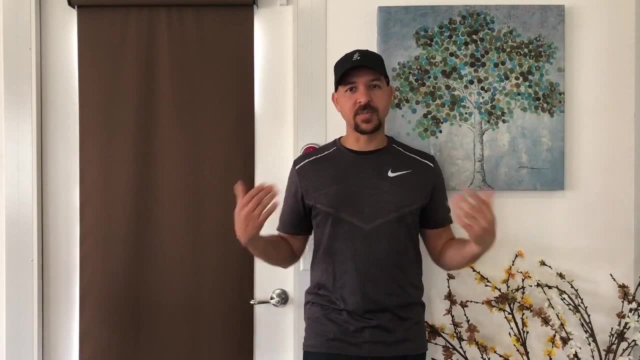 All right guys. so if you're watching this video and if you're not, one of my students, let me introduce myself. My name is Rich Gordon. I'm the band director at Sycamore Junior High School in Anaheim, California. Today's going to be a live video. just some quick rhythm reading. 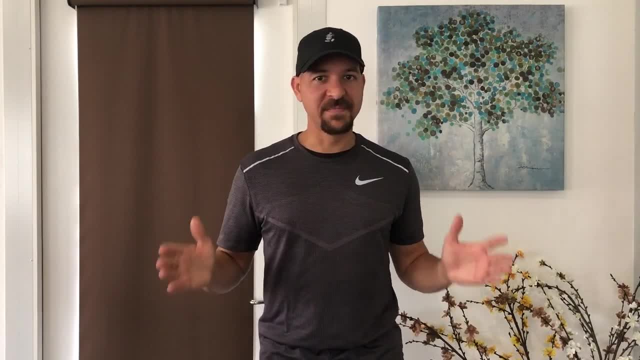 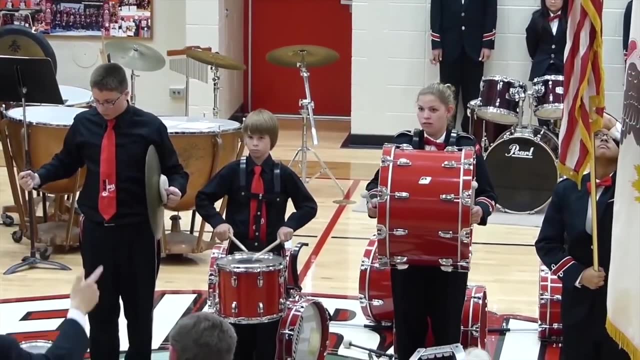 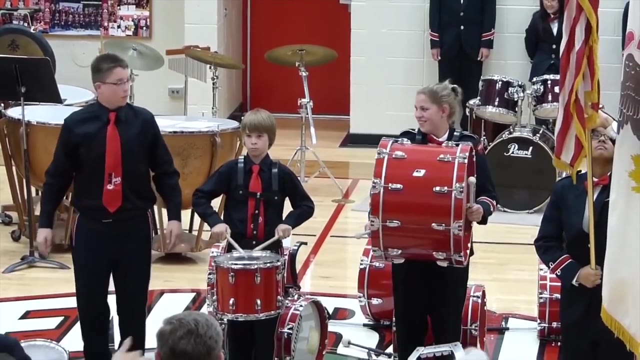 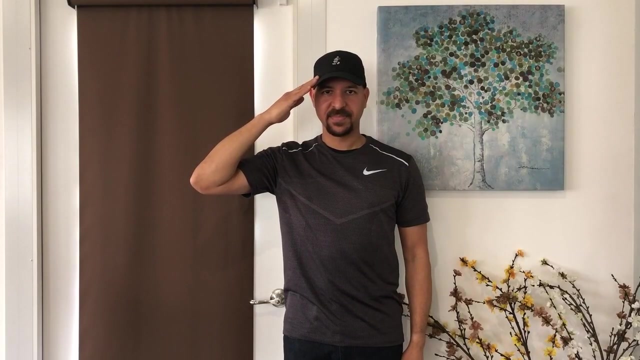 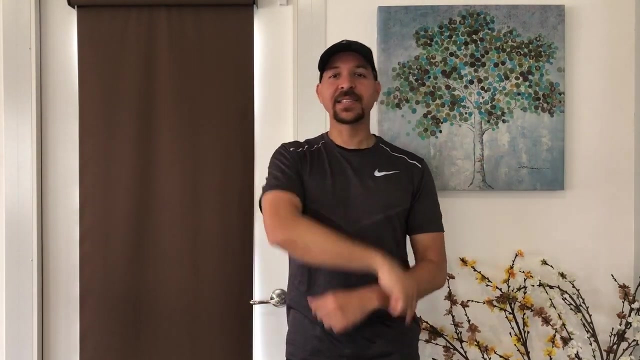 but first let's check out one of my favorite fail videos of all time. Here we go: Classic classic music fail video. All right, guys, let's get right into the rhythm reading. Here is your beginning example, right here. Now take a look at this example. 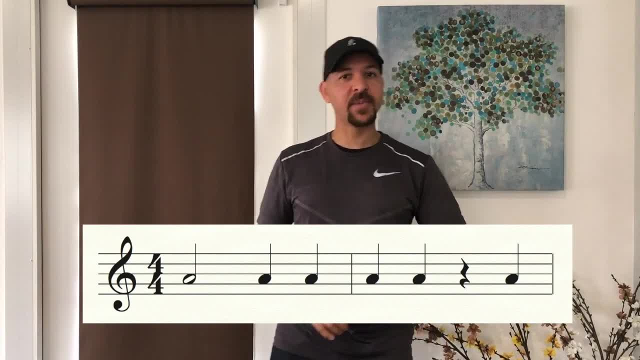 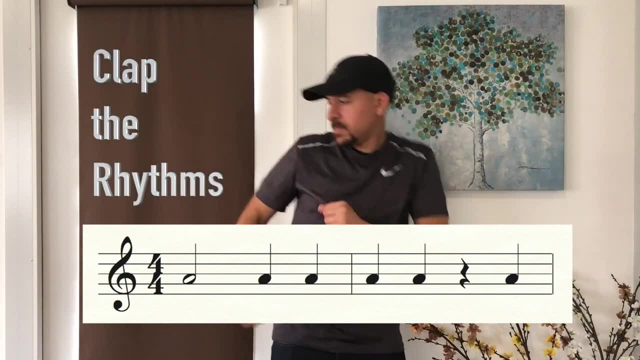 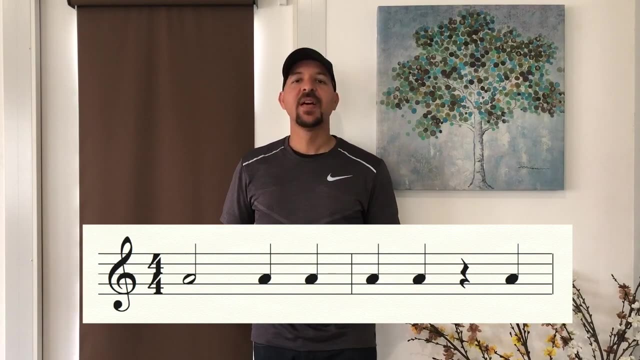 What we're going to do is I'm going to ask you to clap and count out loud. I'm going to give you a beat. so when I tell you to go, you're going to clap with this beat, Feel that beat And one, two ready. go, One, two, three, four. One, two, three, four and stop. Good, All right. 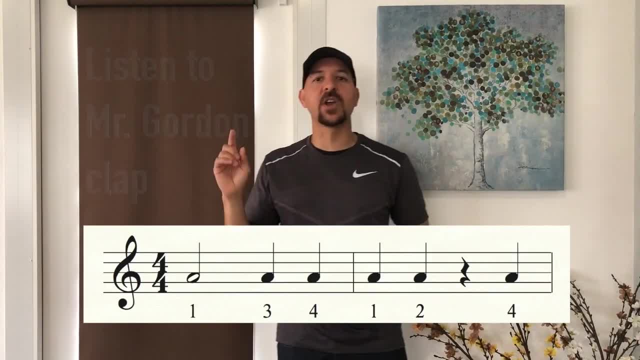 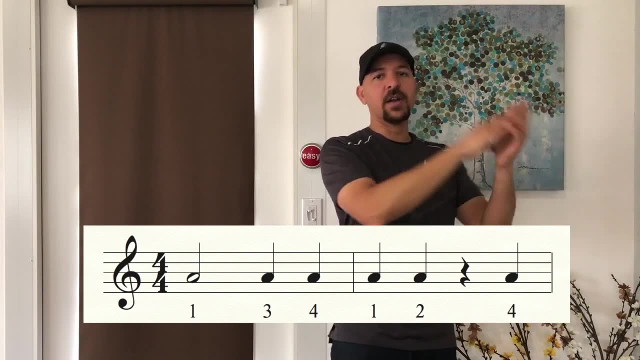 let me clap it for you. I'm going to give you an example of what it's supposed to sound like. Here we go: One, two. I'm clapping now. One, two, three, four. One, two, three, four, All right. 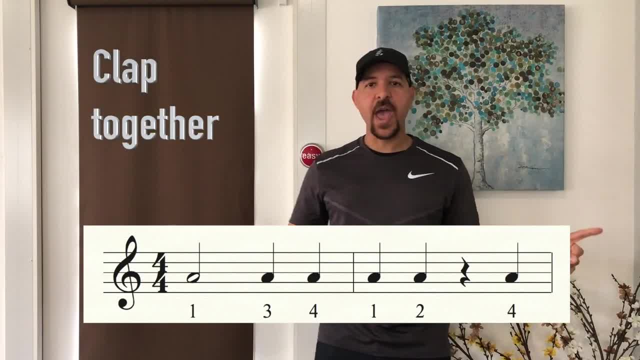 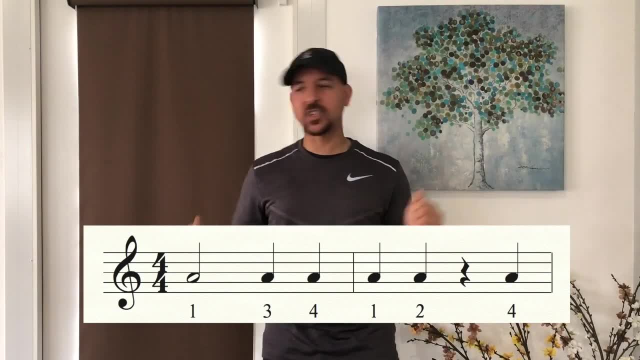 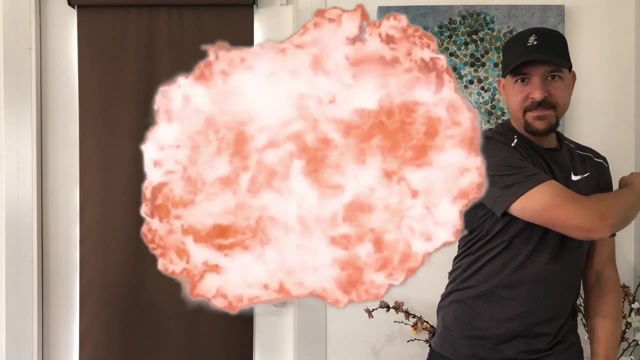 clap along with me. now, Here we go. One, two ready, and one, two, three, four. One, two, three. Alright, ladies and gentlemen, give yourselves a round of applause. That was awesome. That deserves our easy button right here. That was easy. 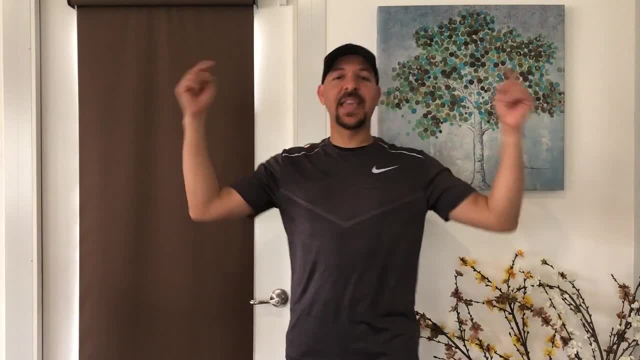 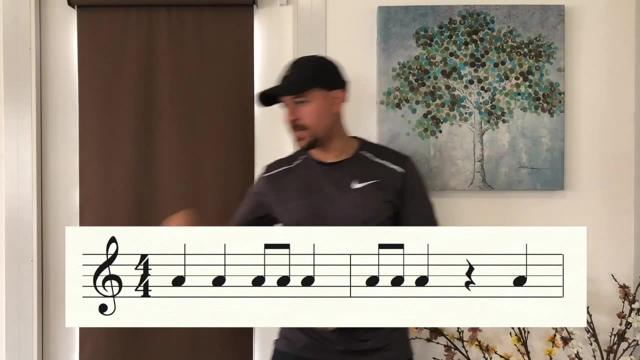 All right, we're going to get straight into our second example. This is the intermediate example, and this example has some eighth notes in it. I'm going to ask you to clap it again. First, I'm going to give you a beat. Feel that beat, okay. 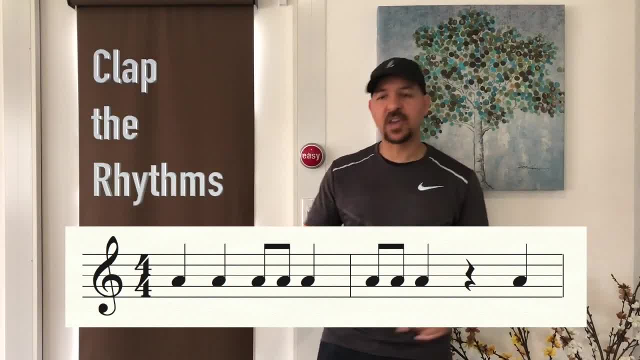 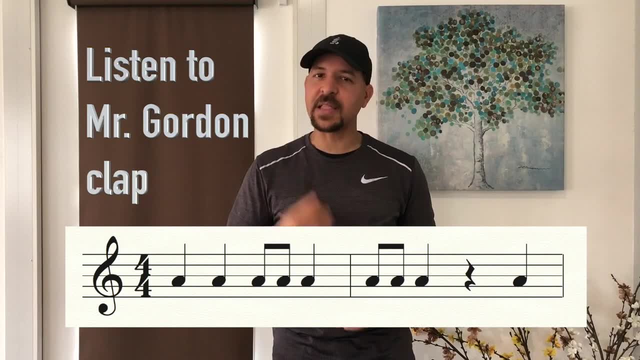 we're going to clap and count out loud: 1,, 2,, ready, go. 1, 2,, 3,, 4.. 1,, 2,, 3,, 4.. And stop, Good, Now listen to me, clap this rhythm for you. I'm going to clap it out loud: Ready, And 1,, 2,. 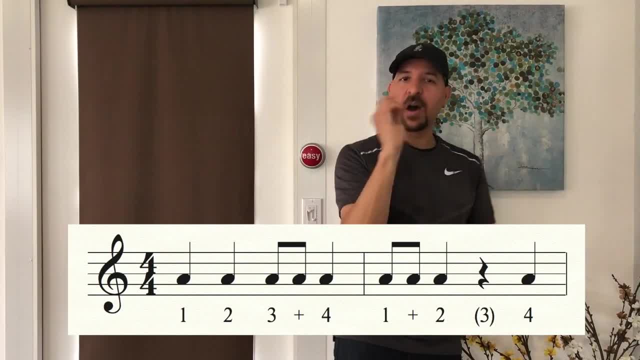 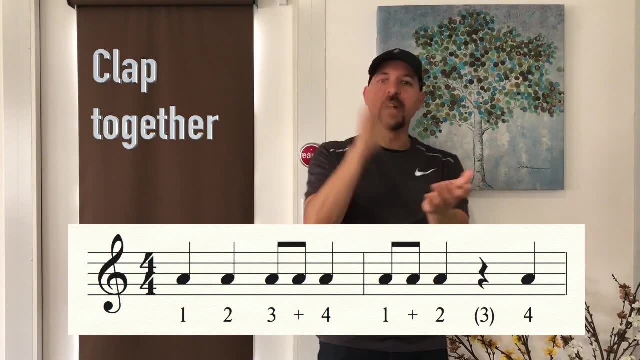 3, and 4.. 1, and 2,, 3,, 4.. All right, your turn again. Clap it along with me. 1,, 2,, ready, go. 1,, 2,, 3, and 4.. 1, and 2,, 3,, 4.. All right, another round of applause for you, ladies and. 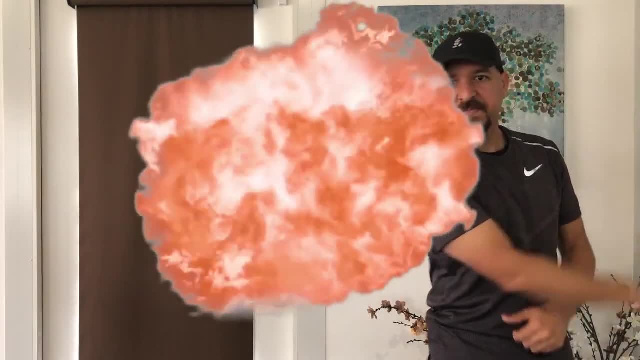 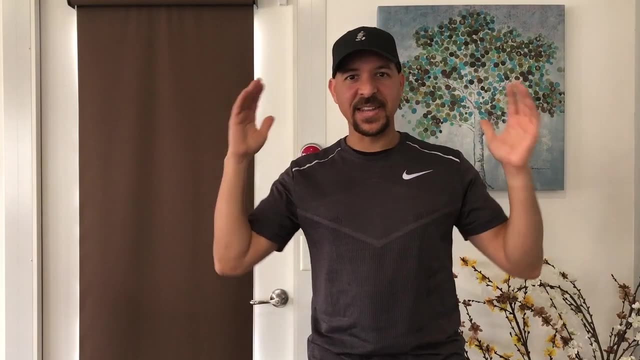 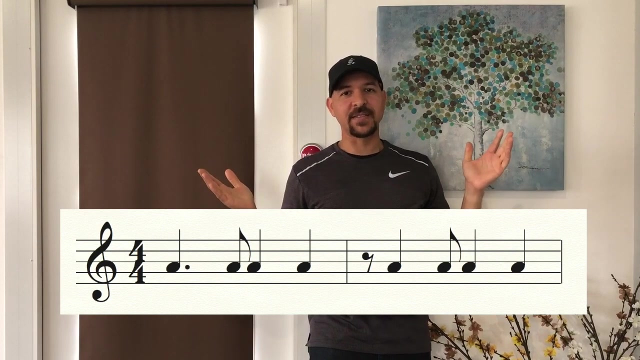 gentlemen, Another easy button. That was easy. All right, ladies and gentlemen, we are almost done. Let's get ready for our third and final example. This is the advanced example. Now, of course, when I say advanced, keep in mind that I teach junior high school. This is pretty. 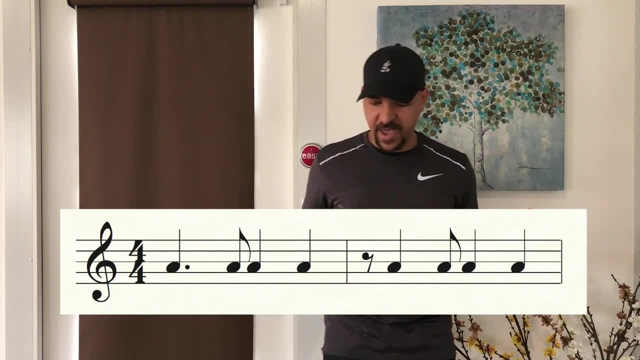 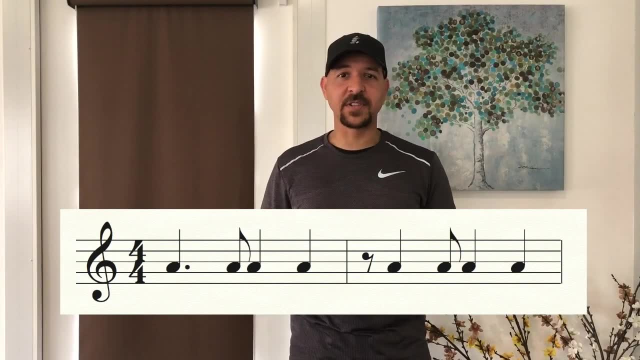 advanced, especially for some of our best students. So let's get ready for our third beginning classes. So this one has some syncopation in it. Syncopation, Obviously: you're going to have to learn how to count off the beat. You're going to have to learn how to 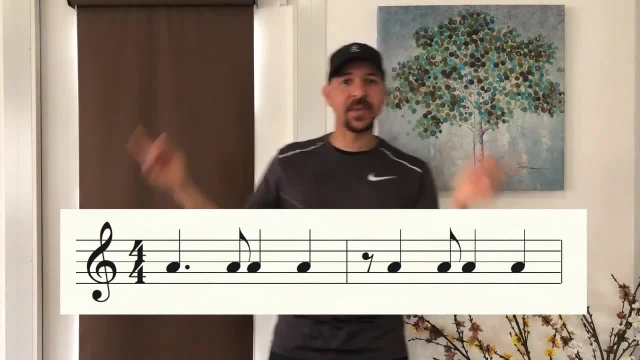 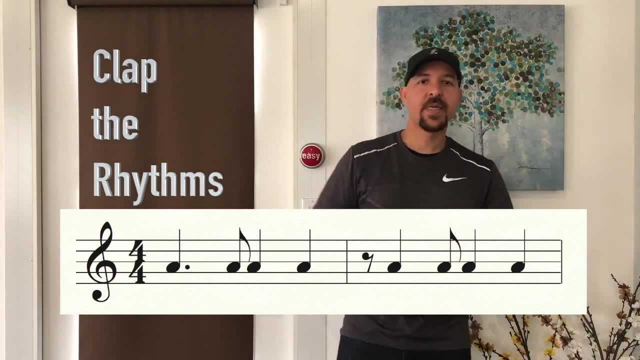 count with those and counts. So take a look at it. You try it. first. Let me give you the beat: 1, 2, ready, and 1, 2,, 3, 4.. 1,, 2,, 3, 4.. And stop, Good, Let me clap it for you. Here's what. 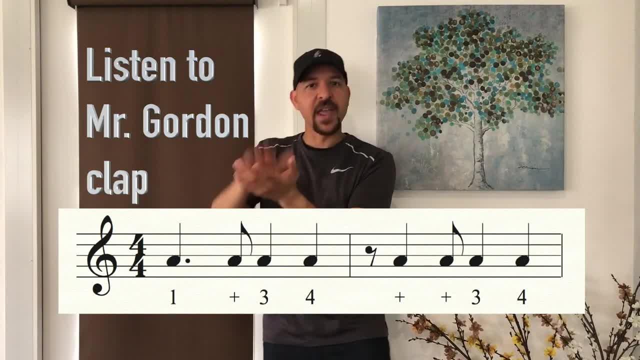 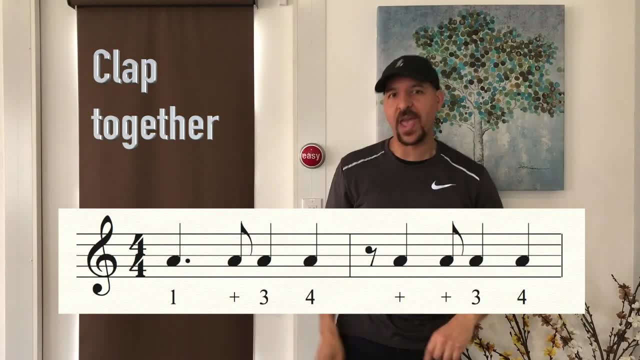 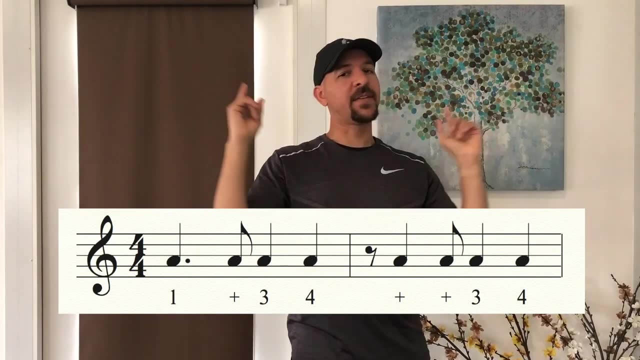 it sounds like Ready, And 1,, 2, and 4.. 1,, 2,, 3,, 4.. All right, let's get ready for our third and final example. Let's try it again: 1,, 2, and 4.. 1,, 2,, 3,, 4.. And stop, All right. 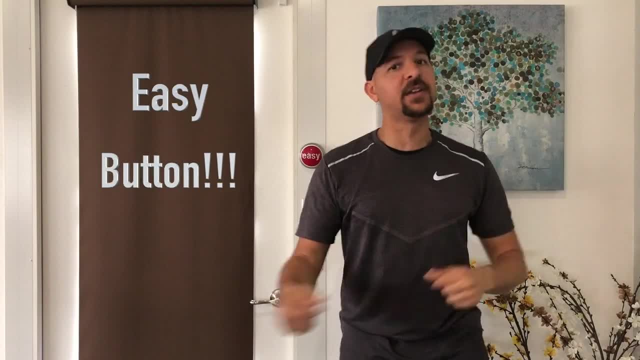 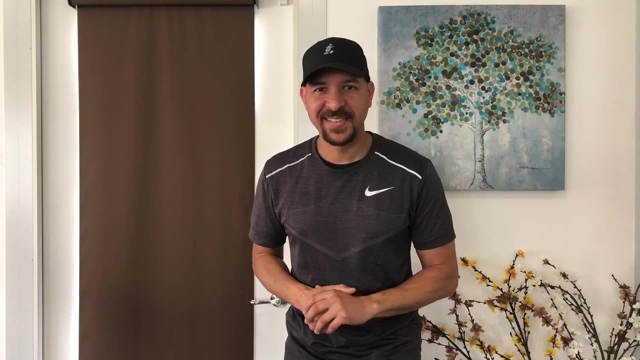 if you got that one, you definitely deserve a round of applause and another easy button. That was easy. All right, that is going to do it for us today. Ladies and gentlemen, you did such a wonderful job. Thank you for staying safe. We'll see you next time. Bye. 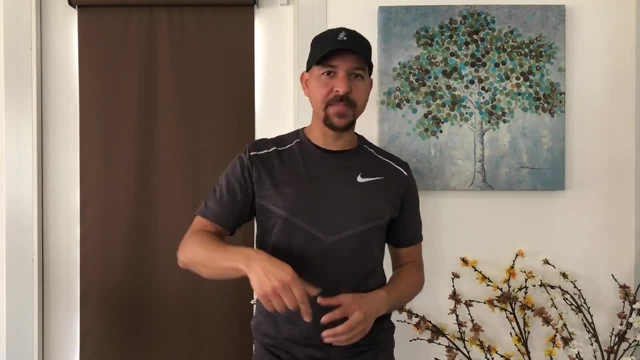 And healthy and happy out there. If you like this video, please subscribe Sycamore JHS Band Videos. Please hit that like button and I'll see you again next time.